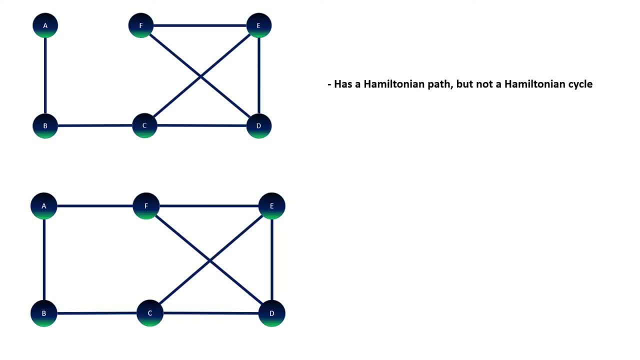 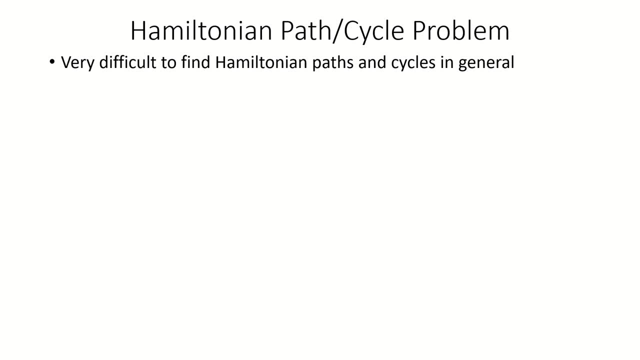 which is the initial vertex. However, not all graphs with Hamiltonian paths have Hamiltonian cycles. The question of whether or not a graph has a Hamiltonian path or cycle is generally very difficult to answer. However, for certain classes of graphs, the question can be simplified by. 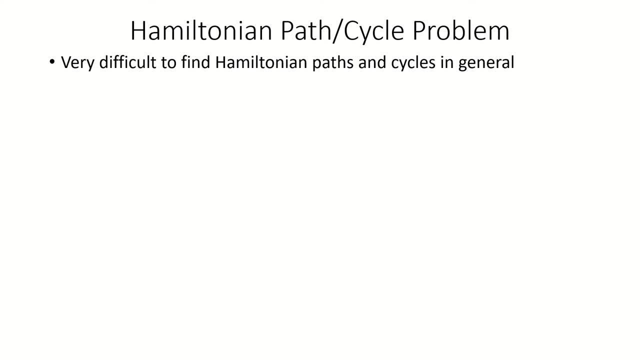 analyzing the structure or devising algorithms for those specific types of graphs. For example, the question of whether or not a grid graph contains a Hamiltonian cycle is very easy to answer, provided you know the length and width of the grid graph. It is proven that if one or both sides of the grid graph are even in length, as in this example, 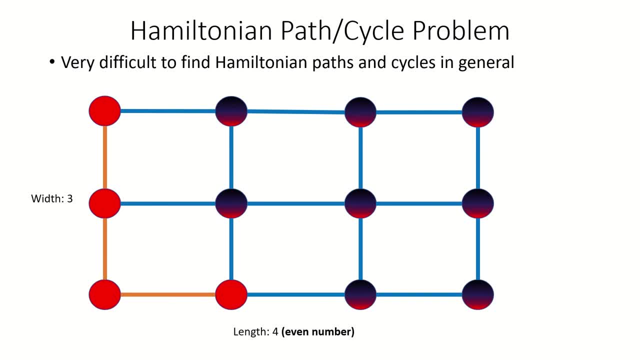 there exists a Hamiltonian cycle in the grid graph, Can you see why There also exist sufficient conditions for graphs of any kind to have Hamiltonian cycles or paths? Here are two of those sufficient conditions. The first is Dirac's theorem, which states that if we 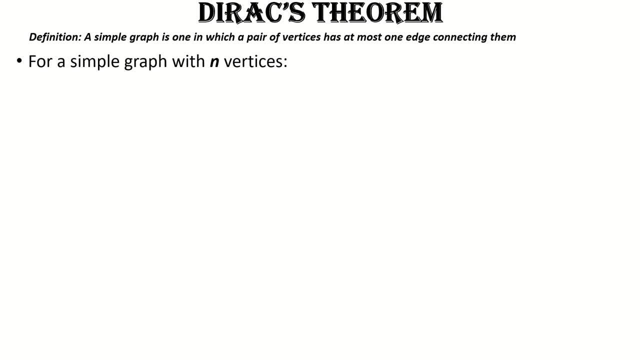 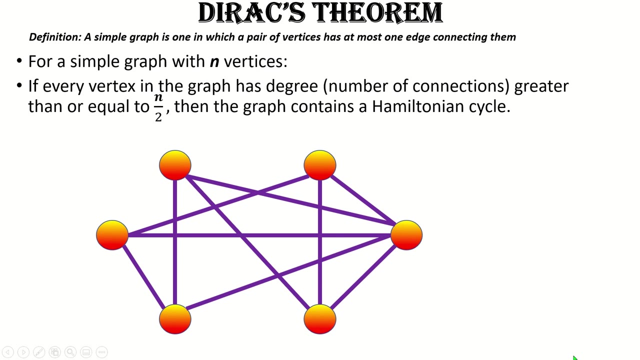 have a simple graph with n vertices where every vertex has degree greater than or equal to n over 2, then the graph contains a Hamiltonian cycle. Here's an example of a graph that, by Dirac's theorem, contains a Hamiltonian cycle. Notice that there are six vertices and every vertex has degree at least. 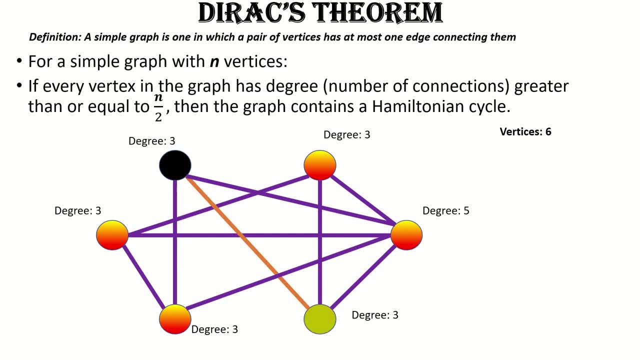 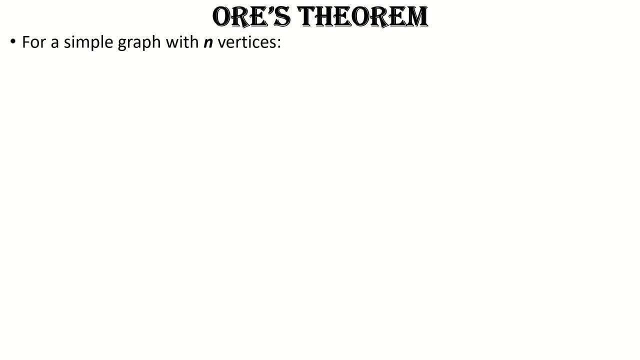 6 over 2, or 3.. Sure enough, there is a Hamiltonian cycle in this graph. Orr's theorem, a generalization of Dirac's theorem, states that if we have a simple graph with n vertices and if, for every non-adjacent pair of vertices in the graph, their degrees sum to at 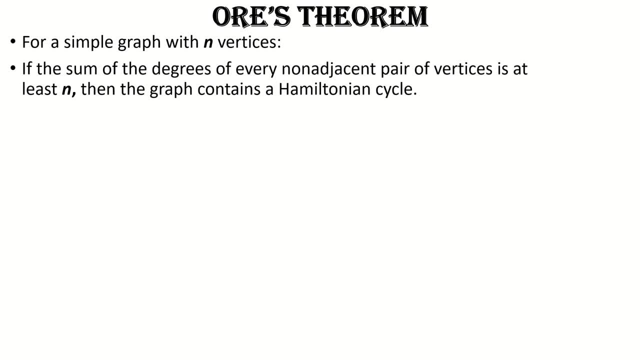 least n, then the graph contains a Hamiltonian cycle. Here's an example of a graph that, by Orr's theorem, contains a Hamiltonian cycle. It has five vertices, and notice that no matter which pair of non-adjacent vertices you choose- and there are only two of them- the sum of their 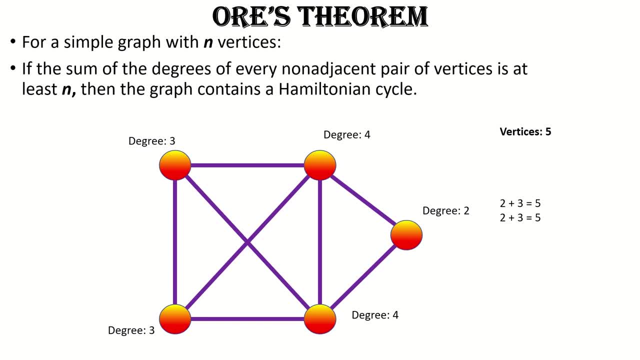 degrees is greater than or equal to 5, the number of vertices in the graph. Here is one Hamiltonian cycle in this graph. Notice that any graph that satisfies Dirac's theorem will satisfy Orr's theorem. Notice that any graph that satisfies Dirac's theorem will satisfy Orr's theorem as it.